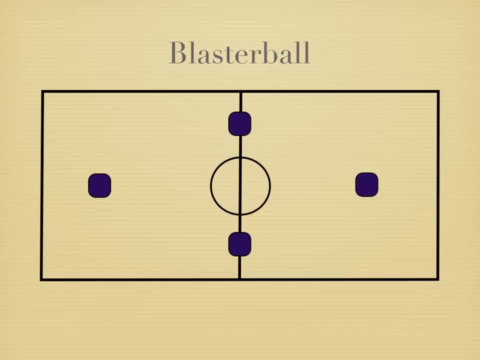 baseball rules, but you're going to be using a lot of the same skills and it's a fun game to play when you're doing a baseball unit. So here we see the batting team lined up along the wall and there's a fielding team out in the field. 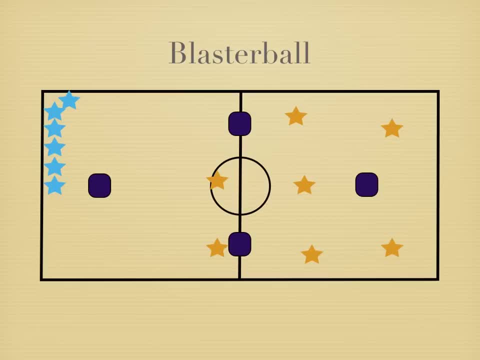 Now the fielding team. they're not necessarily on any baseball positions, so there's no first baseman, second base, third base. In this case, there's not even a back catcher. You can have one if you'd like, but you will have a pitcher who will start with the ball. 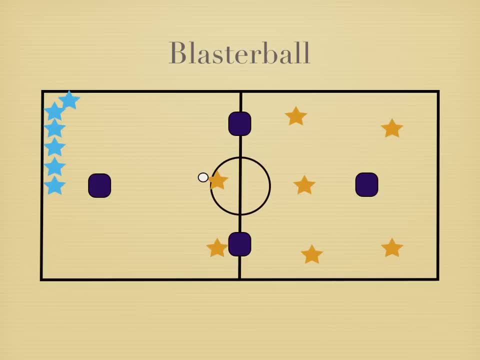 You could also have a tee instead of a pitcher. It's up to you. for, however, you want to work with your class And we're going to take a look first at the batting team. So, basically, the goal of the batting team is to hit the ball. 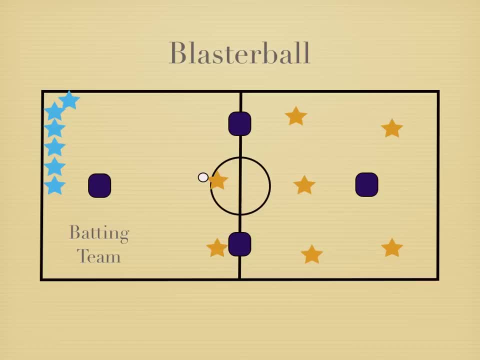 and round the bases. so that's kind of similar to baseball. The only difference is the batting player must round all of the bases without stopping at any base. So the batting player cannot stop once the ball is hit. So here you see, the ball is hit. 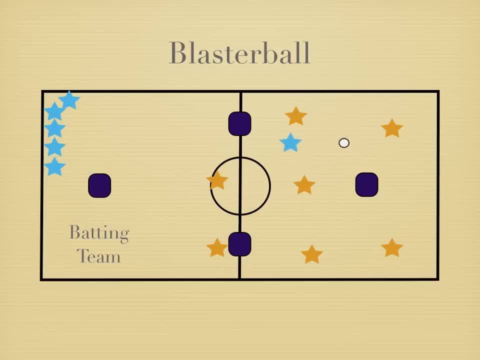 and the batting player must run and cannot stop, just has to keep trying around all the bases and make it home. So they're going to do that before the fielding team does something. Here we're going to take a look at the fielding team. 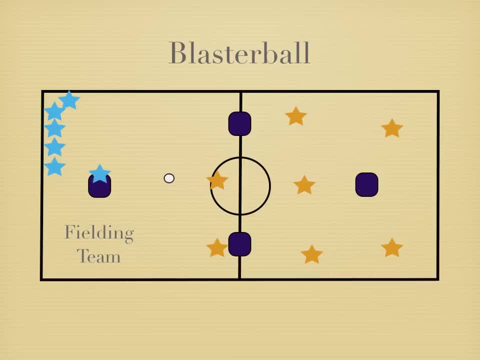 So the same situation. we have our batter coming to plate and the batter has hit the ball. Now you can imagine for a second. the batter is rounding those bases, like in the previous slide, But here the fielding team. what they're going to do is they're going to try and complete. 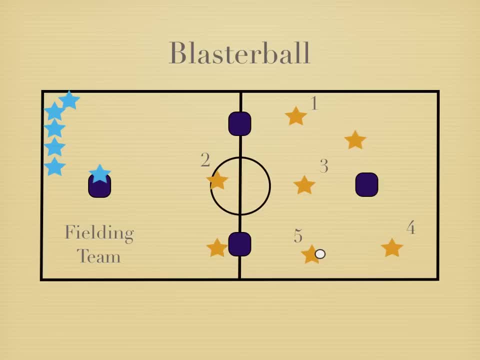 five passes to different people. So it can't be the same person, that pass wouldn't count. They have to do five passes before the runner can round all of those bases. So it's kind of a race between time for the batter to run around all the bases, or 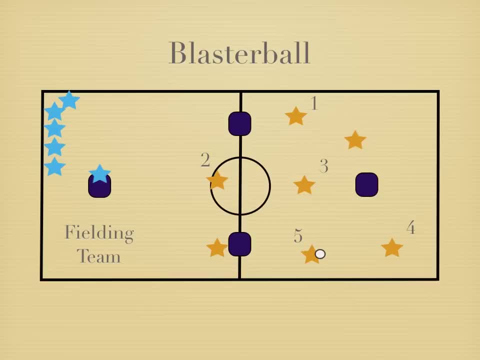 the fielders to make five passes And they want to count them out when they're doing that, And if the runner makes it, they get a point for that team, If not, that runner is out. And if they drop the ball, then again that pass doesn't count and they can continue from. 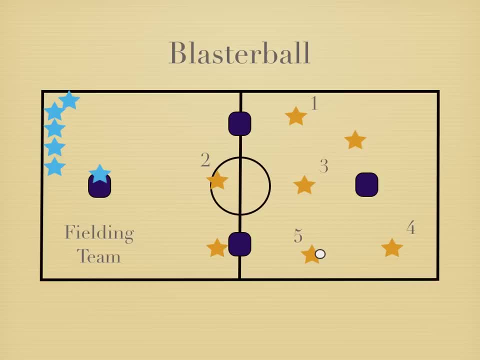 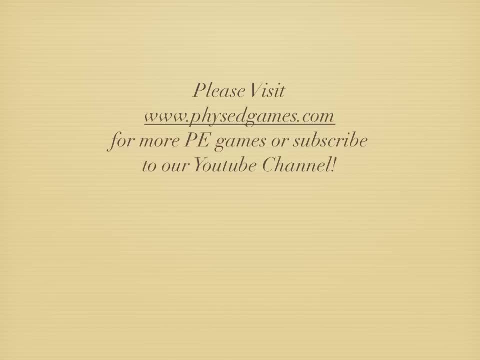 where they were passing And you go once through the order so everyone gets a chance and then switch it up. So that's the basics to Blasterball. I hope you've enjoyed this game. Please head to physedgamescom for more games.